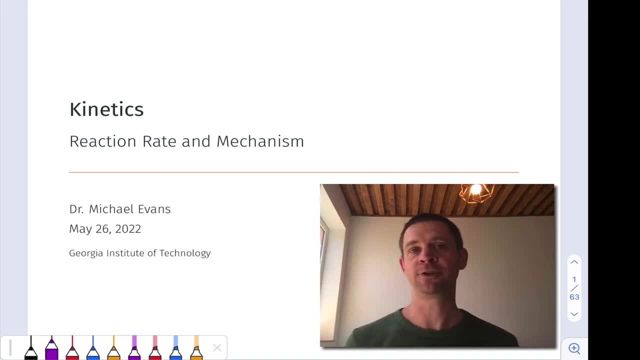 This unit is all about the speed and time dimension of chemical reactions, specifically the field of chemical kinetics. We're interested in the speed of chemical reactions for two reasons. The first is more straightforward: We just want to know how long should we expect a reaction to take? In fact, 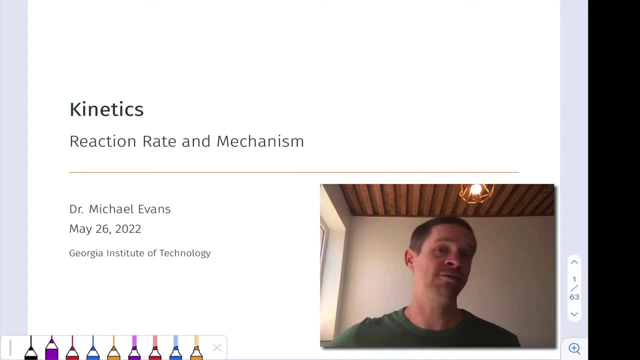 reaction times span a huge range of time scales, all the way down from the nanosecond, microsecond, millisecond scale up to years, decades, centuries, right. And so we want to get a sense of how we think about and express and measure the rates of reactions, so that we know how long a 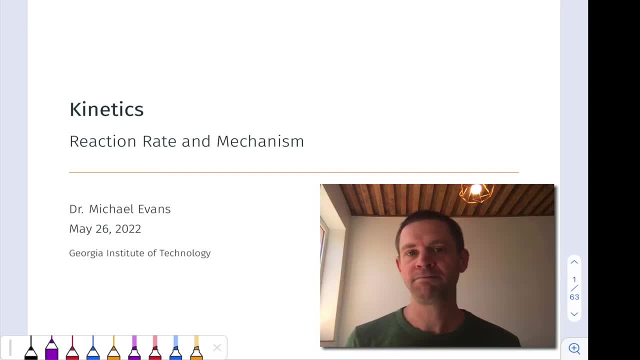 given reaction will take more or less. That's pretty straightforward. The second reason goes a little bit deeper. It has to do with how the reaction actually occurs. What are the bond making and breaking events that occur in the midst of the reaction? 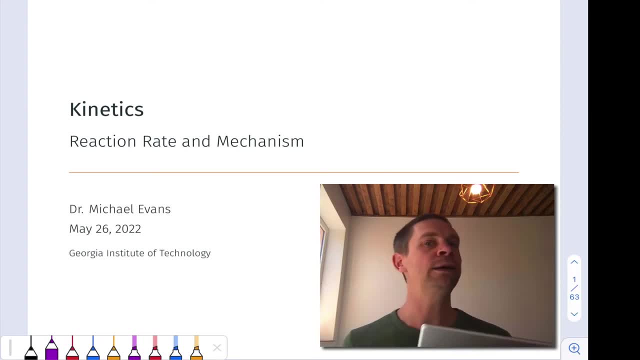 For example, how do atoms and electrons rearrange themselves as the reactants convert to products? Kinetics can give us insight into this as well, and it's what's known as the reaction mechanism, And so toward the end of this unit, we're going to connect reaction mechanism with kinetic data. 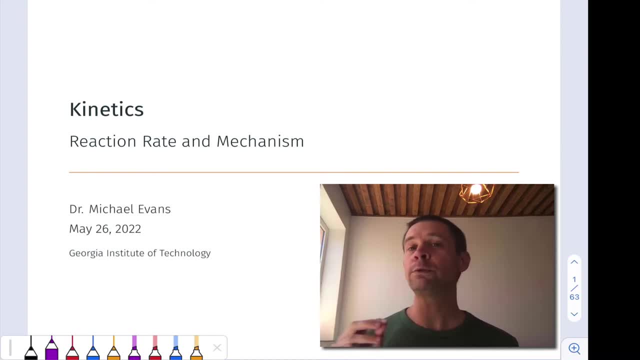 and be able to use kinetic data to distinguish between reaction mechanisms, for example. As you move on to more advanced courses in organic and physical chemistry, you'll see reaction mechanisms again, And the first thing you'll notice is that the reaction mechanisms are not always the same. 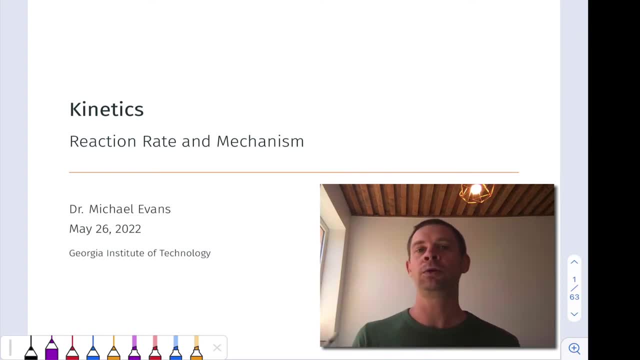 And the first thing you'll notice is that the reaction mechanisms are not always the same And the focus, especially in organic chemistry, is the actual movements of electrons: bonds made, bonds broken, the reactive intermediates involved, so on and so forth. Chemical kinetics is the foundation. 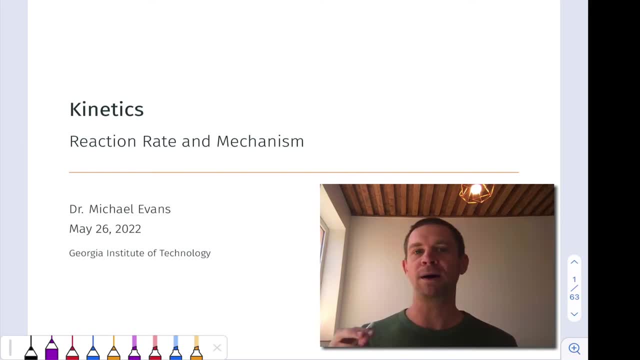 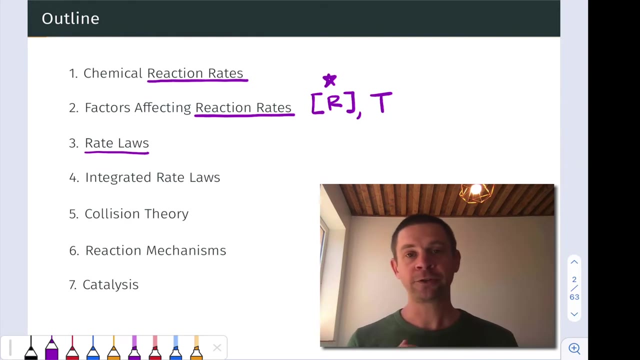 of those theoretical ideas, And so it's worth keeping in mind, And this connection between kinetics and mechanism is a theme throughout your chemical education that will come back again and again. So in this particular unit we're going to look at seven different sections. The first defines what's really the key quantity of chemical kinetics, which is the 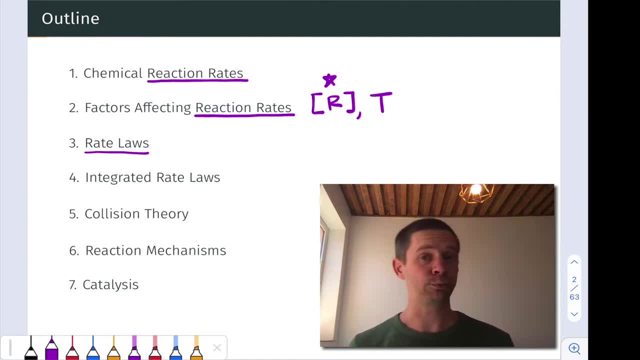 reaction rate. This is a measure of how quickly the reaction proceeds in units of concentration or partial pressure or some other measure of concentration per unit time. So we'll talk about the various types of reaction rates. There's actually a couple of subtleties here and how we 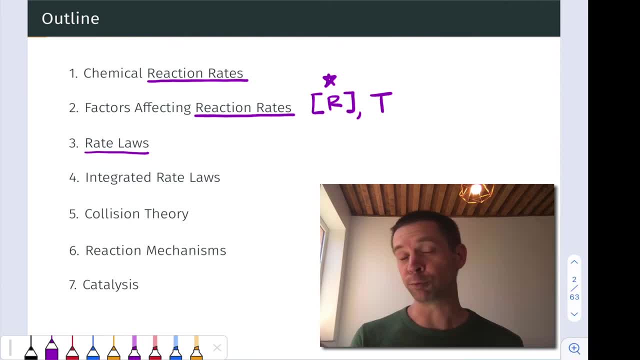 think about those mathematically, the units involved, how we can represent them on a graph and that kind of thing. In the second section we'll look at experimental variables affecting reaction rates, most specifically concentration, the concentrations of the reactants and temperature, And there's some. 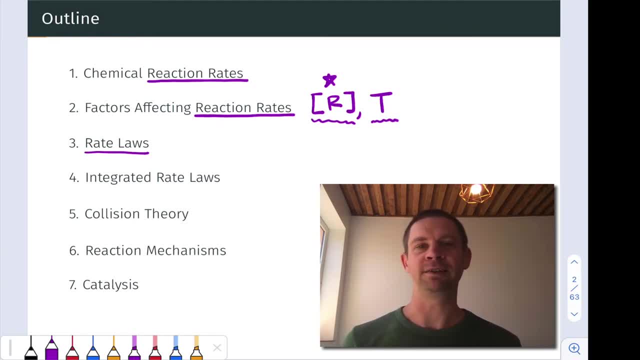 intuitive ideas here that you're probably already familiar with from everyday life. We're going to put a mathematical spin on those intuitive ideas, And the basis of that math is really a theoretical model of the temperature and concentration dependence of the reaction rate And speaking. 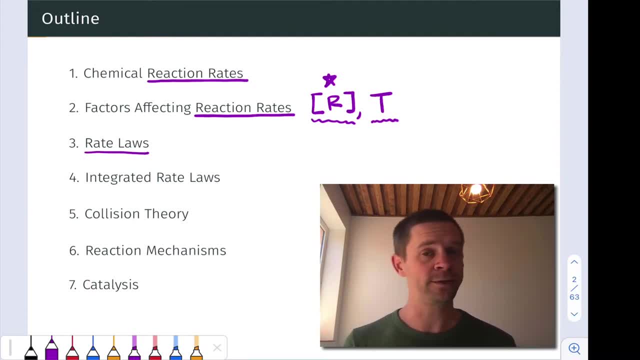 of that concentration dependence. we're going to look at the temperature and concentration dependence of the reactants, which are typically more important in themath of Valentine's Law and U invites. that's the focus of the third and fourth sections. in the third section We're going to 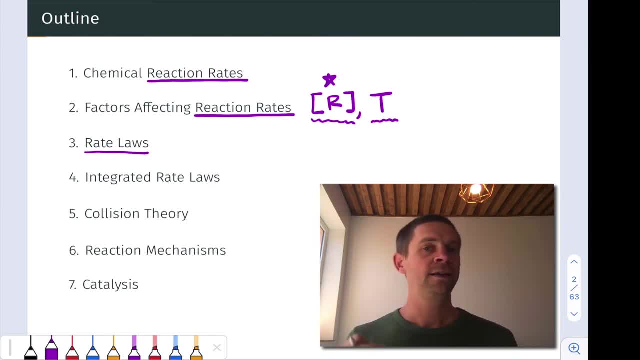 introduce the concept of the rate law or differential rate law, which relates the reaction rate expressed as a derivative to the concentrations of the reactants raised to powers times a constant called the rate constant, And we'll explore the math behind that and what the rate law can tell us and how we can apply the rate law in that. 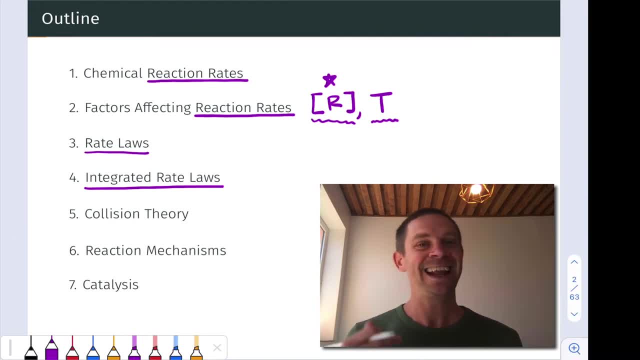 section rate law and integrate it to give the integrated rate law. And the integrated rate law, as complicated as it sounds, is simply the concentration over time, the time dependence of the concentration of a reactant. That's what the integrated rate law is, nothing more, nothing less. It's what we expect. 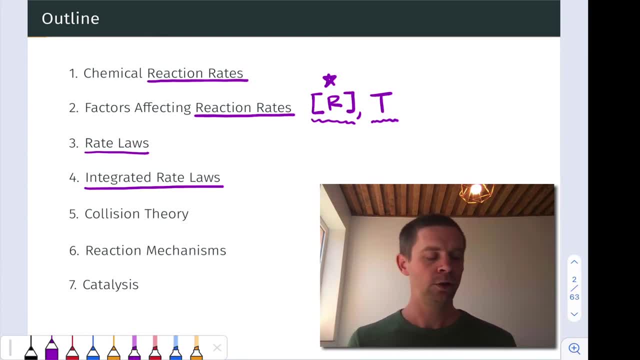 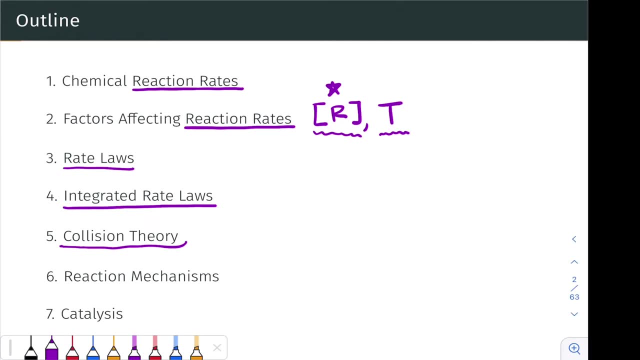 a graph of concentration versus time to look like for a chemical reaction. Collision theory is a theoretical molecular model that underpins how we think about chemical kinetics, why it's temperature dependent, why it's concentration dependent. In section six we'll make that. 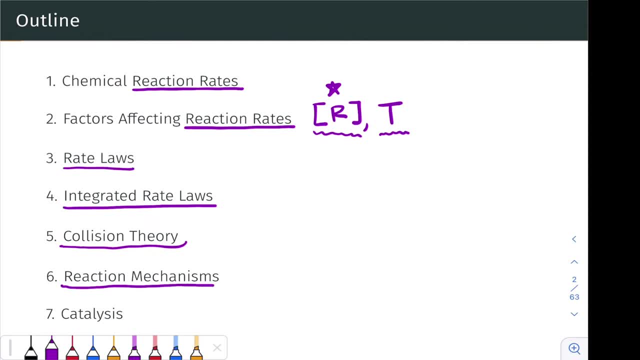 connection between the reaction mechanisms and kinetics, beginning to understand how we can use kinetic data, specifically the rate law, to distinguish between possible mechanisms. And in section seven we'll look at the very important concept of catalysis, this idea that a relatively 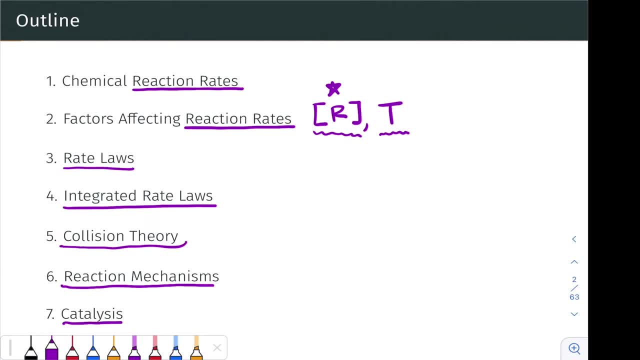 small amount of a substance can be a reaction to a reaction, And in section seven we'll look at the very important concept of catalysis, this idea that a relatively small amount of a substance can accelerate a chemical reaction by modifying its mechanism and lowering the activation energy of 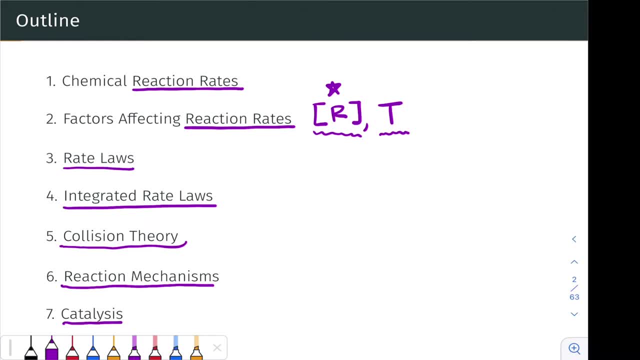 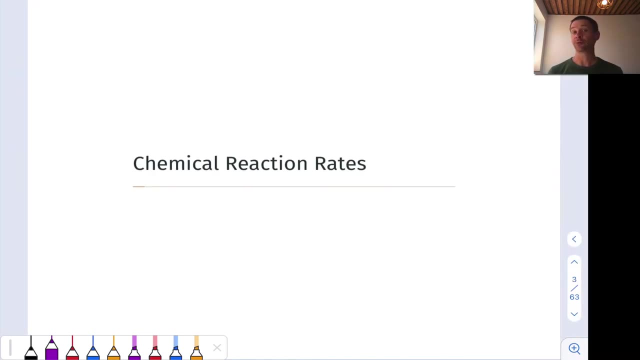 the reaction. This is a very exciting and very active area of current research, because accelerating chemical reactions obviously gives us access to valuable products in a relatively short time frame. Let's begin by defining what we mean by the chemical reaction rate and look at the various 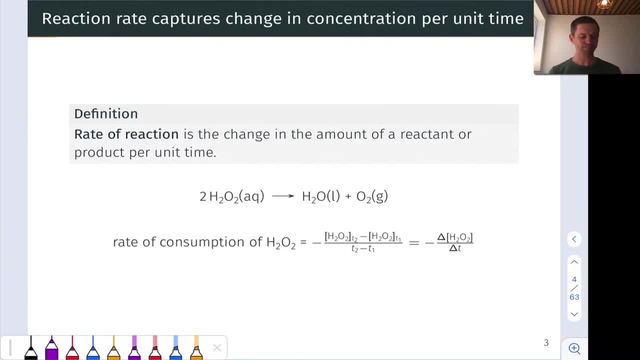 places where chemical reaction rate pops up. Let's begin by defining what we mean by the chemical reaction rate and look at the various places where chemical reaction rate pops up. Let's begin with a definition for the rate of reaction. Rate of reaction is the change in the amount of a reactant or product, or change in. 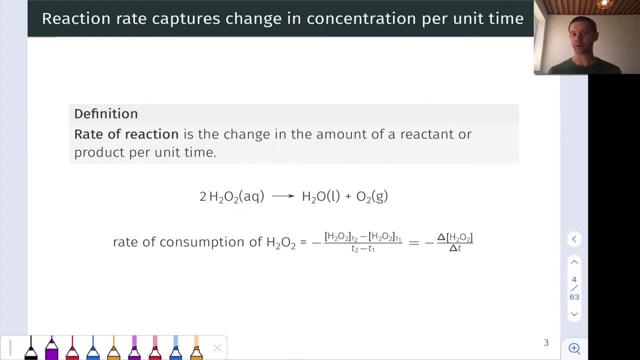 concentration of a reactant or product per unit time. And this quantity is positive by convention. and this is worth keeping in mind because as we think about change, we can think about a concentration increasing or decreasing and generally, if we're looking at a product, for example, coming in, the reaction rate will naturally be positive. 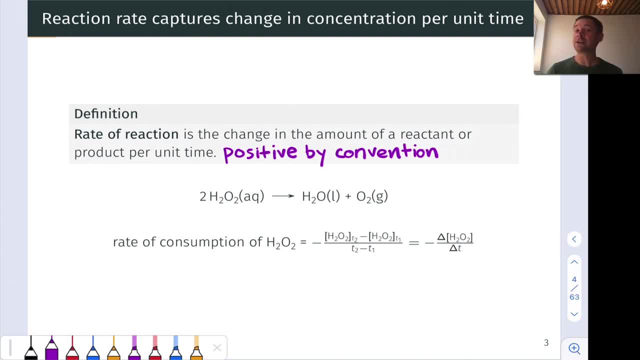 If we're thinking about a reactant disappearing, however, the change in concentration is negative, but a negative sign is used to ensure that the rate of reaction is positive by convention. So take, for example, the reaction you see on this slide: 2H2O2 in the aqueous solution goes. 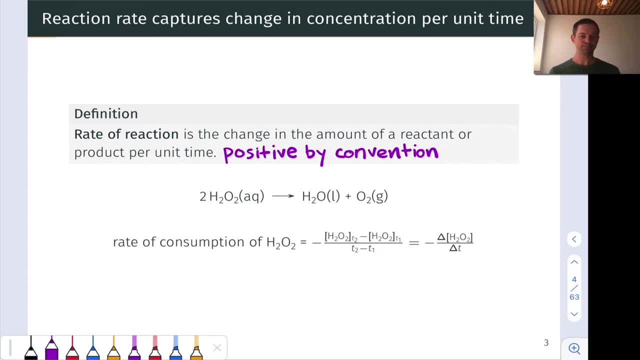 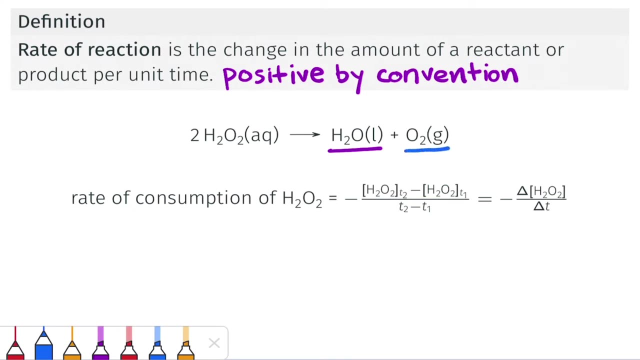 to H2O liquid and O2 gas, And we can think about reaction rate or rate of reaction in terms of any of these three species. For example, we could think about the rate in terms of H2O appearing or in terms of O2 appearing or in terms of H2O2 disappearing, For example, the rate of consumption. 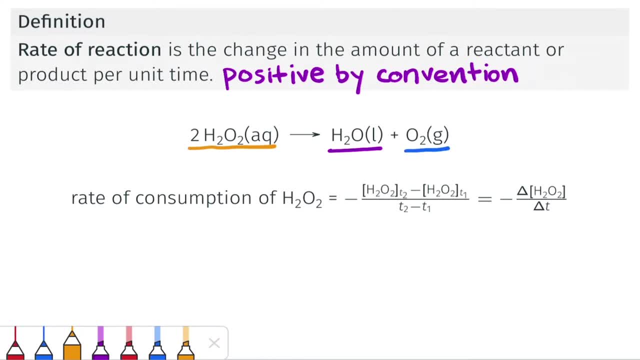 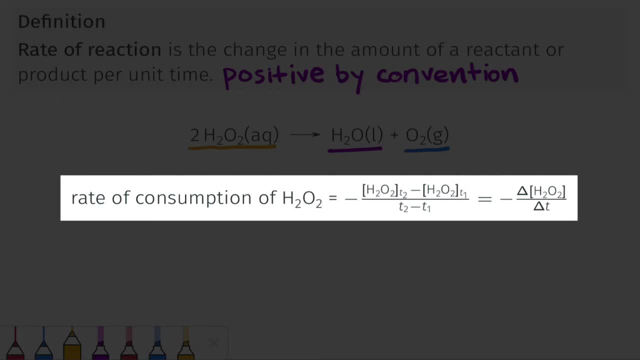 of H2O2 between two time points- let's call them T2 and T1, is equal to the negative of the H2O2 concentration at T2 minus the H2O2 concentration at T1. This is a change in the concentration of the H2O2 between those two time points. 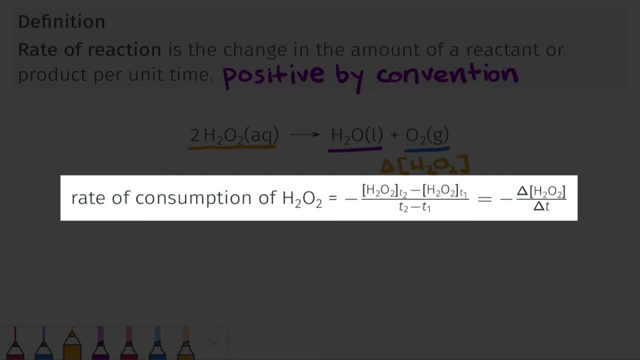 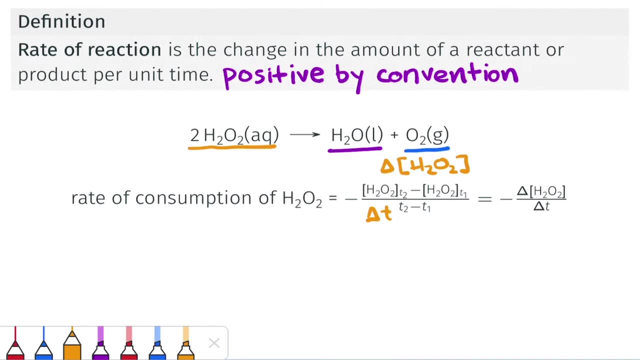 divided by T2 minus T1.. And this, of course, is a change in time between the two time points. So rate is a change in concentration divided by a change in time. Notice that in this example we have a change in concentration between the two time points. 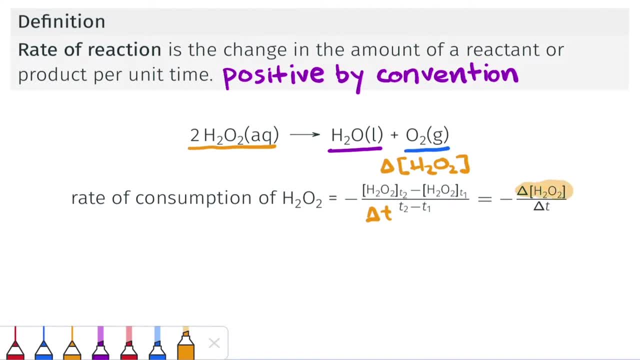 that here. because H2O2 is a reactant, this delta- H2O2 is a negative value- has a negative value. H2O2 is disappearing because it's a reactant. as the reaction proceeds, We can also express the reaction weight in terms of the production of H2O or the production of O2.. So analogous reaction. 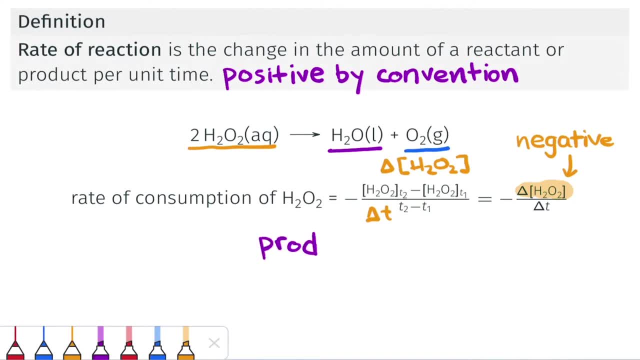 weight expressions could be written, for example, for the production of H2O, by writing the change in the concentration of H2O divided by the change in time, or for the production of O2, as the change in the concentration of O2 divided by the change in time. These are all reaction. 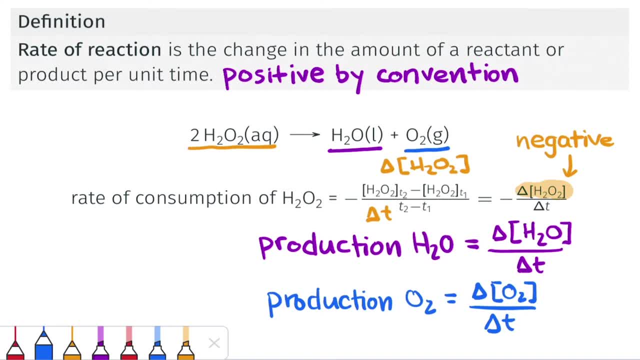 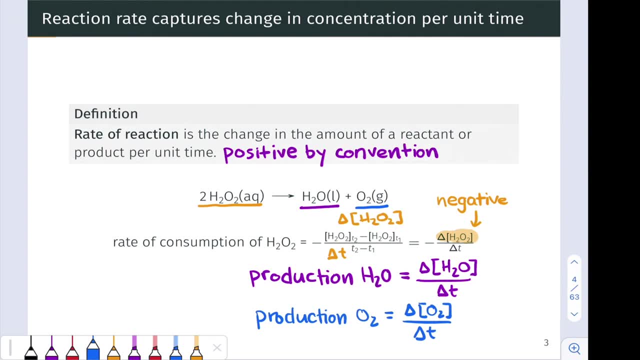 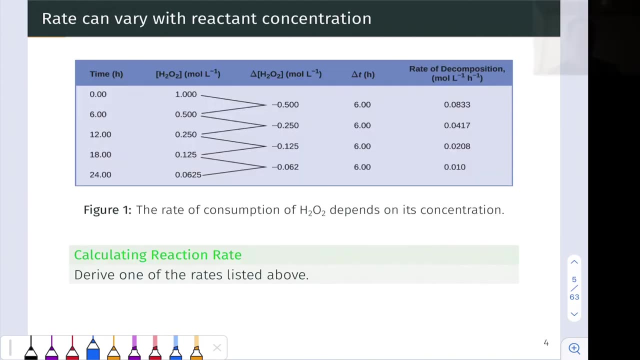 rates, and they're not necessarily numerical, They're not necessarily equal to each other, for stoichiometric reasons that we'll dig into here in a second, but each of these we could think of as a measure of the rate of a reaction. It's a change in the amount or concentration of a reactant or product per unit time. Now, 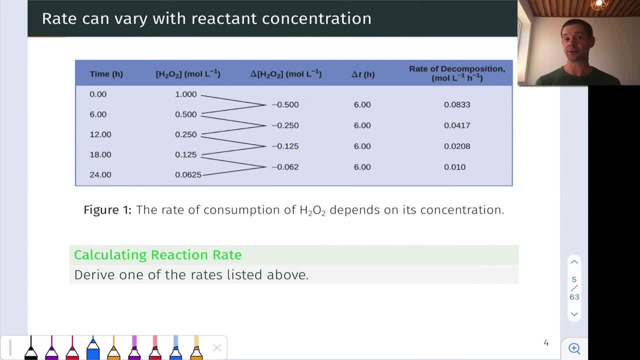 weight often varies with reactant concentration. We alluded to this earlier. Concentration is one of these factors that affects reaction rates. So as a reactant disappears, for example, we may see the reaction rate change And we see that in this table. Notice that the reaction rate, the rate of decomposition, 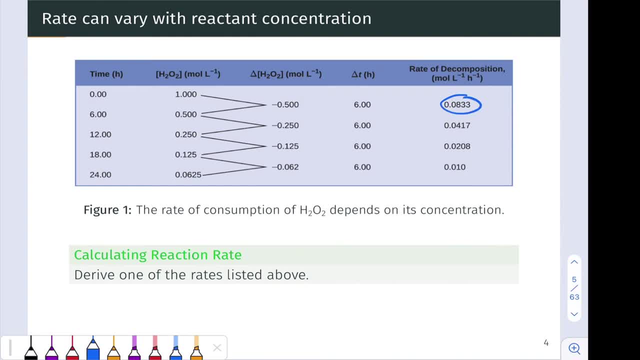 is different early in the reaction, when we have quite a bit of H2O2 there, than later in the reaction, where most of the H2O2 has gone. Let's derive one of these rates of decomposition listed on the right-hand side of this table using the data that's given. So let's look. 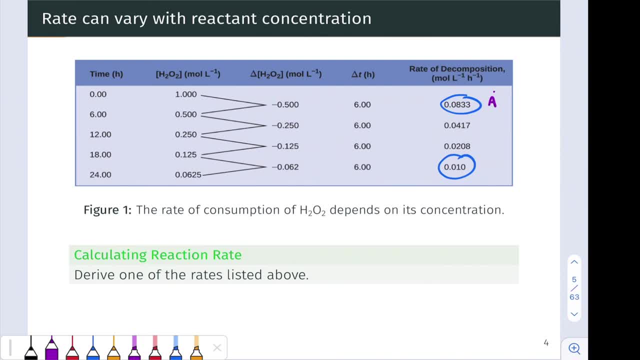 for example, at this rate, 0.0833 moles per second. Moles per liter per hour. Notice the units first of all before we dig into this. Moles per liter per hour. the units of the rate A change in concentration. moles per liter. 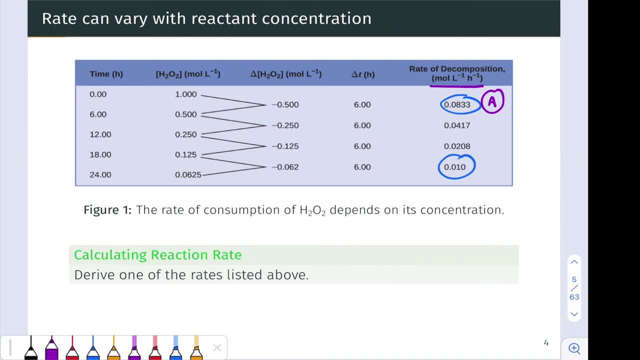 per time per hour. So looking, for example, at that rate which we've called A, we can write the rate of decomposition of H2O2 as a change in concentration divided by a change in time And notice this number's going to come out negative. So what we should do is